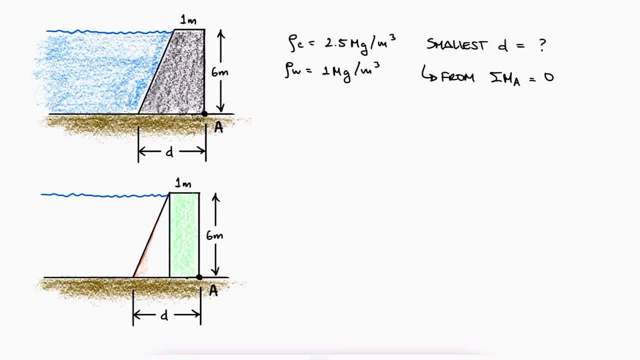 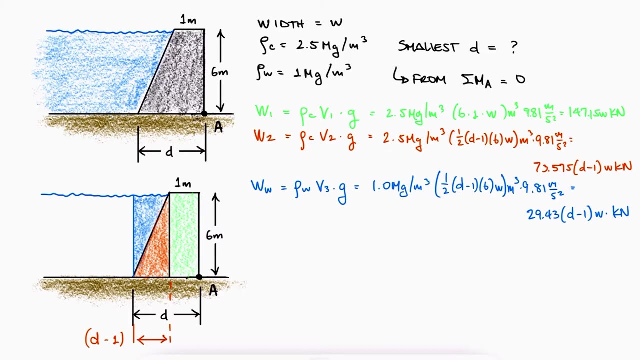 to be zero. The weight of the dam can be divided into two sections, with each weight being the density times the volume times G. The same is true for the weight of the water above the inclined surface, of course with the density of the water, not the density of the concrete. Finally, the 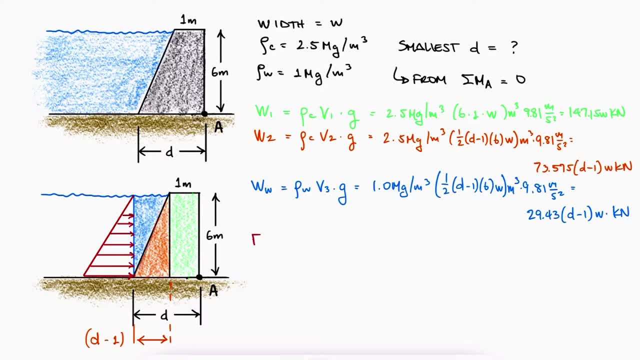 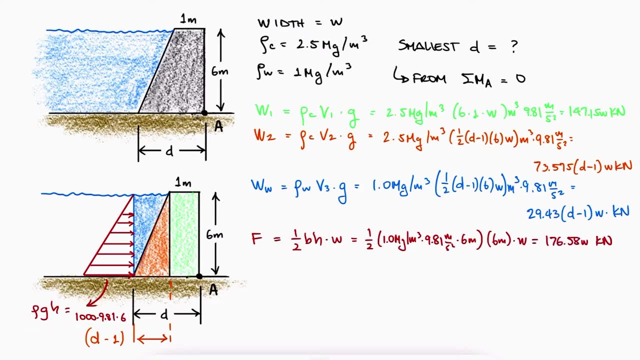 horizontal force caused by the fluid pressure forces of the water above the inclined surface has a total magnitude of its area times the width where the base is the pressure, 6 meters below the water level. The location of all four forces will be at the centroid of each shape. The sum of 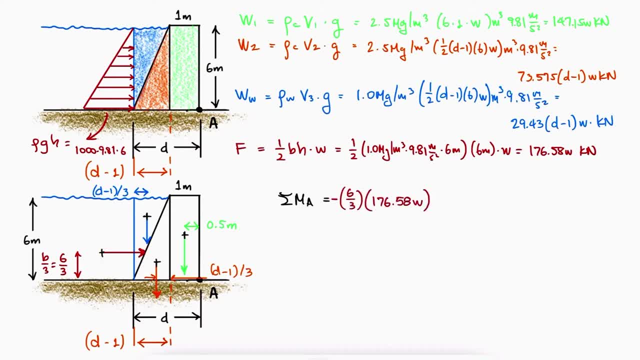 moments will therefore be a clockwise moment for F and a counterclockwise moment for W1,, for W2,, which is located at 1 plus D minus 1 over 3, and a counterclockwise for the weight of the water. 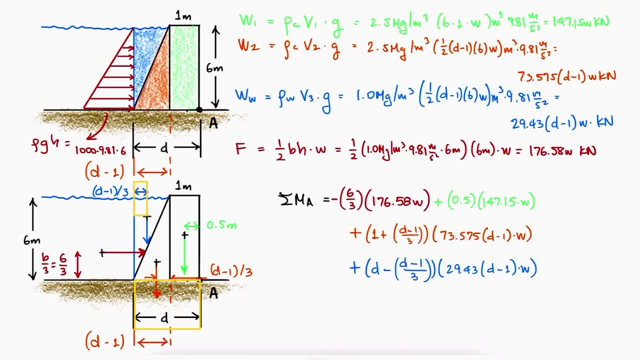 which is located at D minus 1 over 3.. The width dimension cancels out, which is the width of the dam, that we don't see in that third dimension and we solve for the dimension D The link to more fluid pressure. examples as well as: 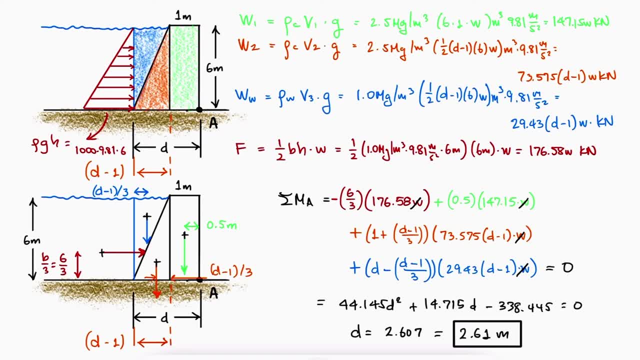 the other main topic. videos from the static scores are found in the description below. Thanks for watching. 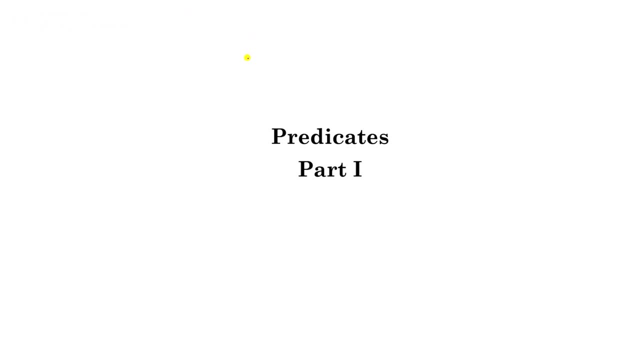 Hello everyone, In this lecture we will understand predicates. First we will define a predicate, Then we will discuss why we are stating predicates. So look at this sentence. I am talking about a general English sentence. Look at this, This part, shaker. this is the subject, and 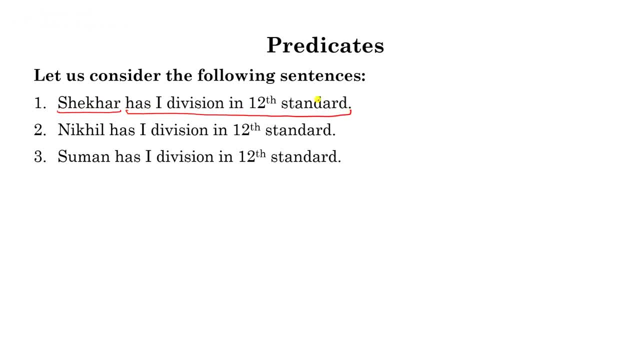 this part from S to standard, this part is predicate. So if you look at this part, this part is telling something about subject. So this part which is telling something about subject is called predicate. So predicate means which is the part of the sentence which